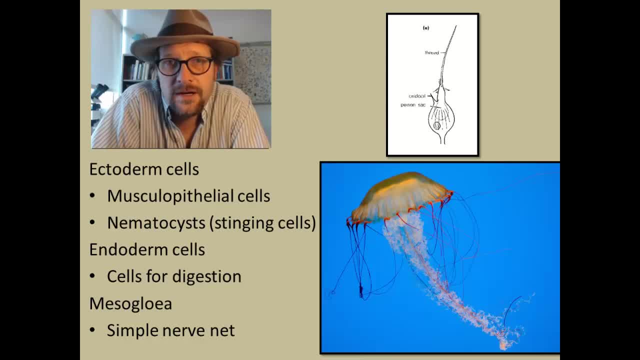 are the stinging cells. The endoderm cells are the cells with poisonous fluids used for protection and food capture. The mnemo cells contain a hair trigger, nidosil, which releases a thread attached to a poisonous sac which can harpoon prey and drag them into the mouth-anus cavity. 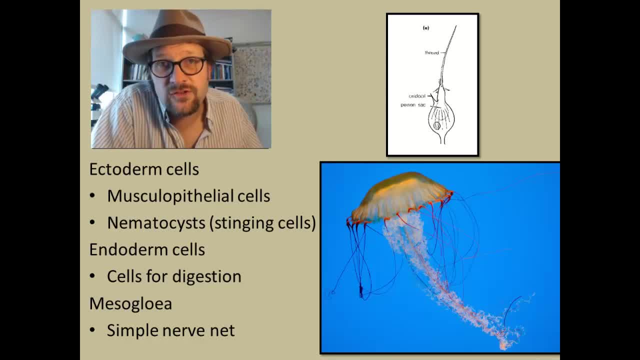 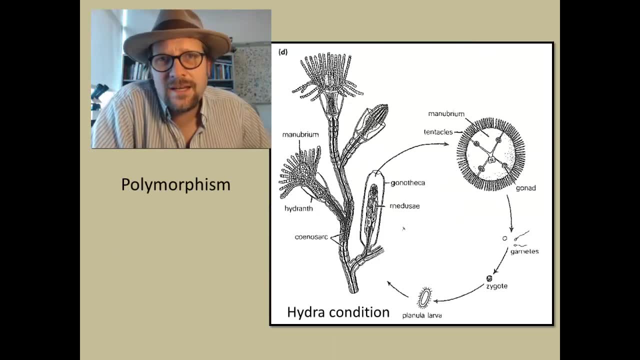 The inner endoderm layers serve the role of digestion and are expanded into radial partitions to maximize the surface area. One of the most fascinating aspects of cnidarians is their complex lifestyle, which is called polymorphism. In the basic life cycle of a cnidarian, the sessile polyp gives rise to 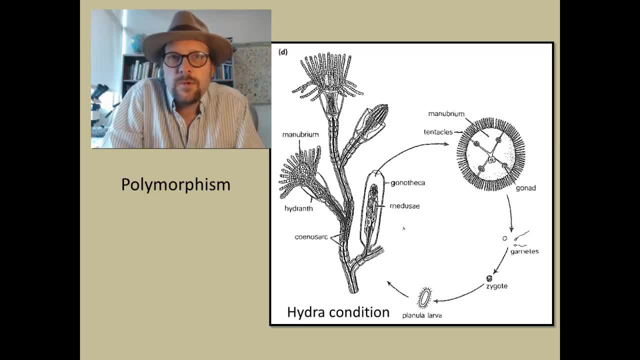 free-floating medusa. through asexual reproduction, The medusa reproduces with other medusa sexually to produce a zygote, which then produces a larvae, then becoming the sessile polyp. Polyps feed by facing upward Medusa. feed by facing upward Medusas. feed by facing upward Medusa. 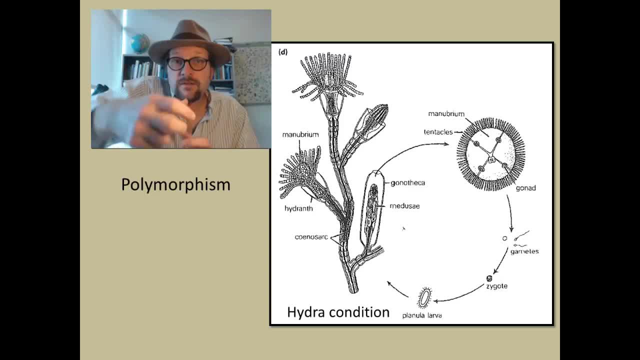 feed by facing downward Medusa feed. by facing downward Medusa feed. by facing upward Medusa lead. by facing downward. A typical jellyfish is the medusa stage, while corals are the polyp stage of the life cycle. Some groups forgo either the medusa stage or become completely sessile, or the polyp. 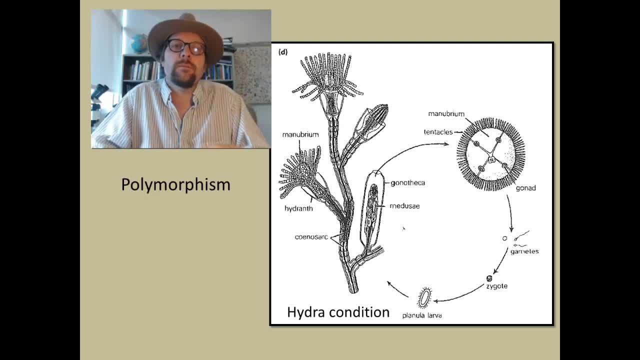 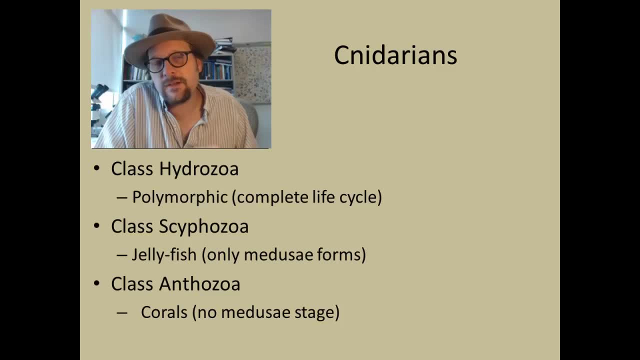 stage and become completely mobile, while others retain polymorphism and have both types of forms. The phylum Cnidaria is split into three classes. The hydrozoan, known from the pre-Cambrian to recent, retain both life stages, both the 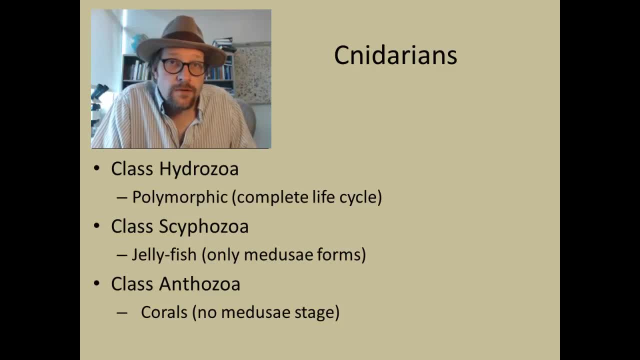 polyp and medusa stage. The scaphozoa, also known from the pre-Cambrian to recent, retain only the medusa stage and include many jellyfish. The anthrozoa, also known from the pre-Cambrian to recent, retain only the polyp stage. and. 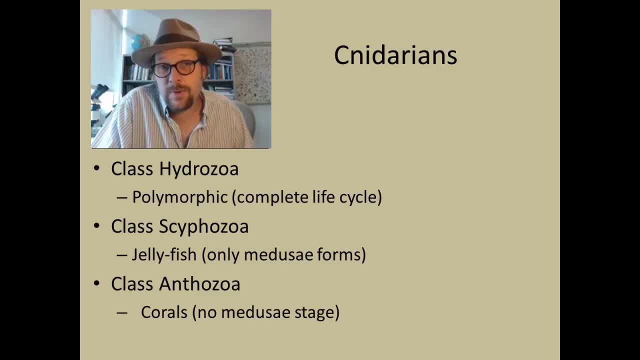 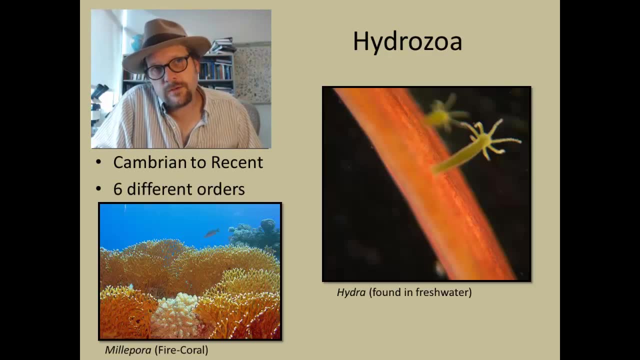 include corals, sea anemones, gorgions and sea pins. Let's take a look at the first group, the hydrozoans. The two best known modern members of the hydrozoa are the small freshwater pond hydra belonging. 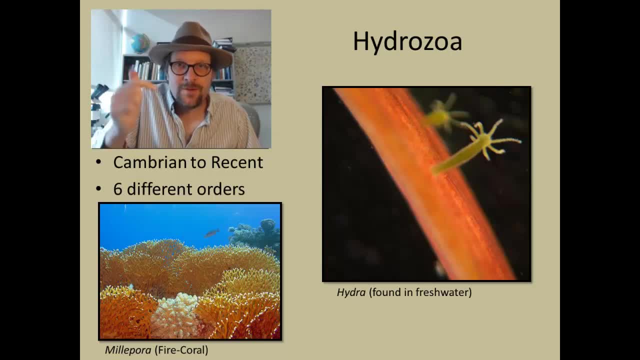 to the order Hydraeidae and the fire coral Myliopoda belonging to the order Hydrochloriana, The Hydrochloriae form, skeletons out of chitin and, as such, lack an extensive fossil record, although there are several symbiotic forms known to live within calcareous tubeworms. 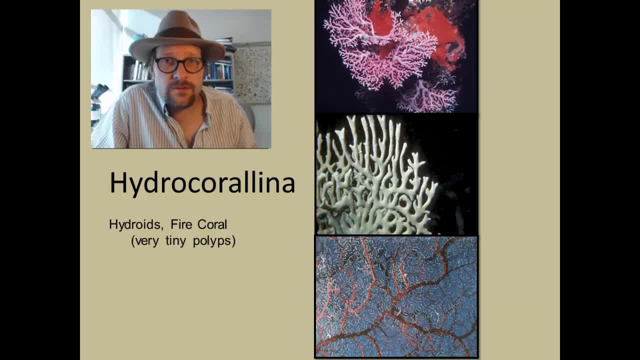 The Hydrochloriania. the fire corals form chalcareous skeletons and can be an important reef builder. The modern fire coral Myliopoda has three types of zooids. Zooids are individual multicellular animals that live within a colony. 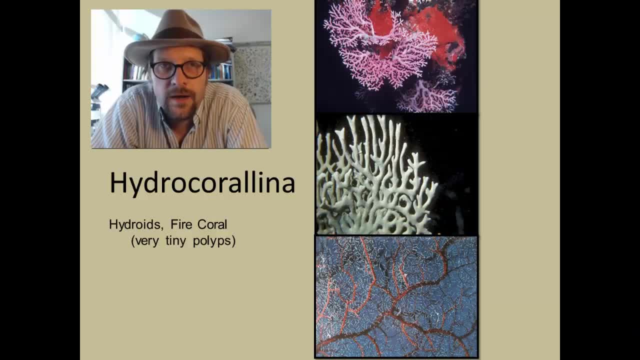 The first type are the gastrozoids that feed, which are surrounded by the didactyl zooids, which have extensive nemosis, poisonous stingers used to capture prey, and the ampulla which can be found in the water, which are released in the water and reproduced sexually by releasing 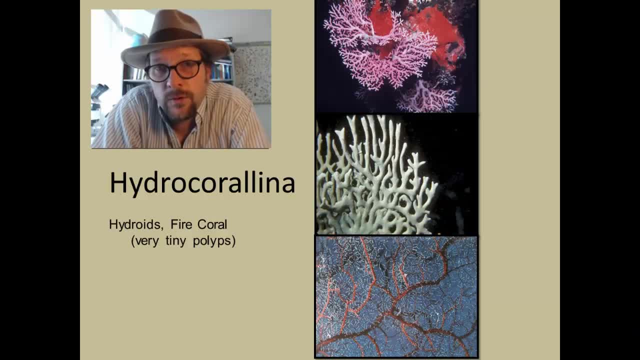 either eggs or sperm to produce small larvae that form new fire colonies. These are where Myliopoda gets its name, which means millions of spores, in reference to all those medusas that are released by the polyps. Zooids can also form by asexually budding, which allows for the colonies to grow over. 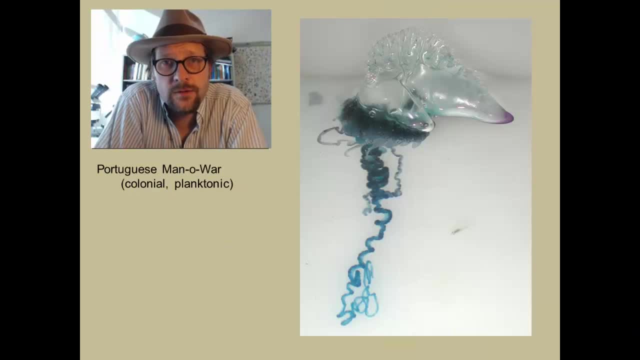 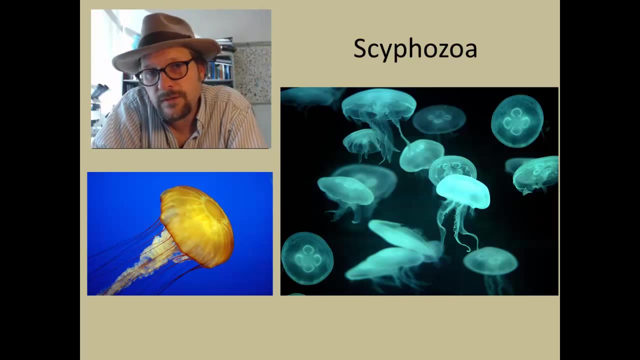 time. Another well-known member of the Hydrozoa is the Portuguese man-of-war, which is a colony of zooids that are planktonic and highly poisonous, with numerous nemosis. The class Scalphozoa includes the jellyfish and retain just the medusa stage of the life. 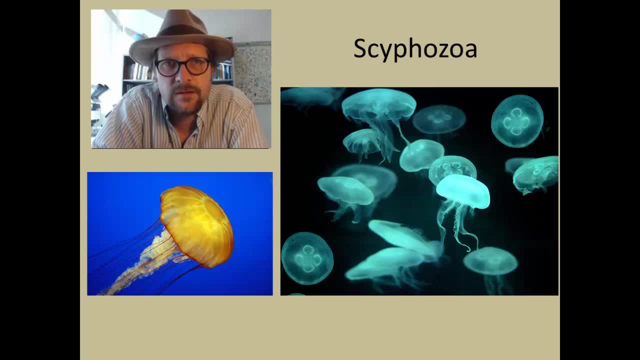 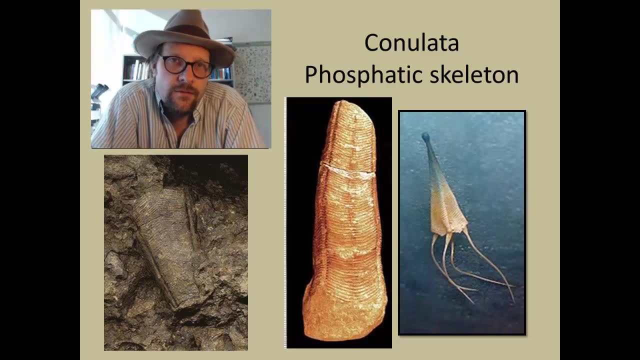 cycle. Jellyfish rarely fossilize since they lack any hard skeleton and only are preserved as body impressions. One unique group of Scaphozoa are the Polyps. They are the conioletes or coniolarids, which are strange pyramid shaped fossils composed 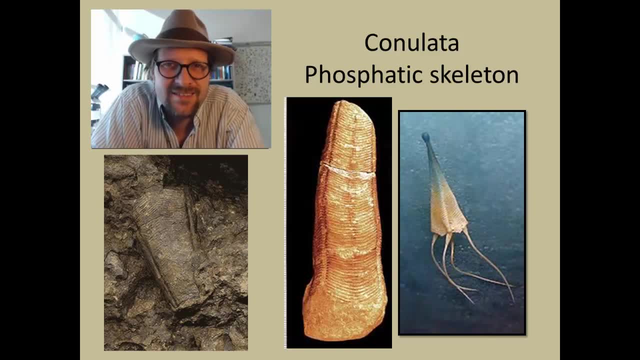 of ridges, of phosphatic skeletons that look like upside down ice cream cones. These fossils appear to be Scaphozoids due to the presence of tentacles and the fact that they are planktonic and being found in deep marine facies by floating around in the 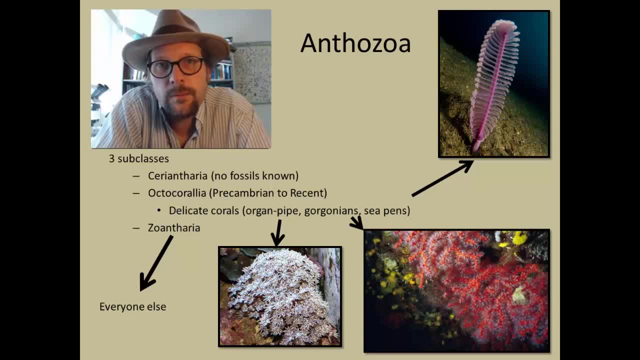 ocean. The Hydrozoa includes cnidarians with only the polyp stage of the life cycle and lack any medusoid stage. They include corals, sea anemones, gorgons and sea pins. The polyps can produce both eggs and sperm, which fertilize into new generations of polyps. 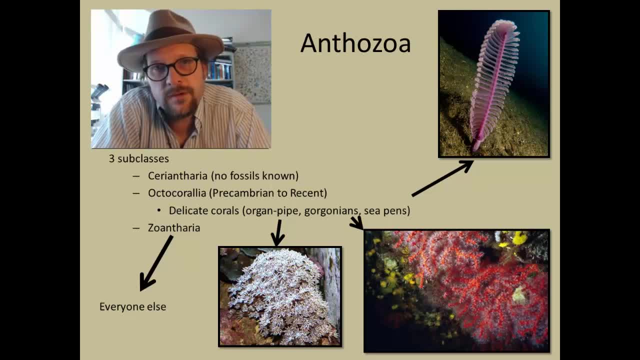 Anthrozoan polyps are much larger in size compared to the smaller polyps of hydrozoans. There are three subclasses of Anthrozoans: 1. The Ceranthrea, the Octochorea and the Zooanthrea. 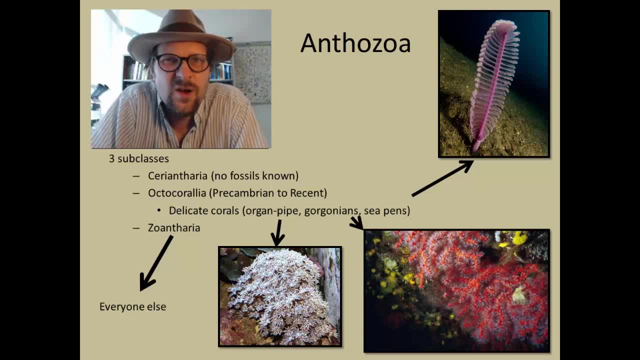 The Ceranthrea lack hard skeletons and such are not known from the fossil record. The Octochorea are corals that have polyps that have an eight-fold symmetry. They are supported by gelatinous coating, with some forming a skeleton with calcareous. 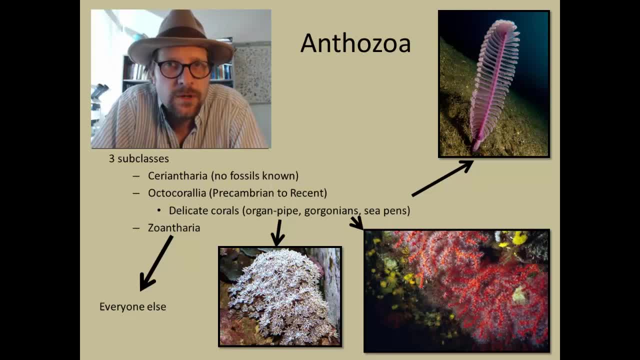 spicules, A few secrete enough calcareous spicules to be recognized in the fossil record, but they are fairly rare. The most common fossil record is the Ceranthrea. The Ceranthrea are a member of the zooanthrea, which are often called stony corals because 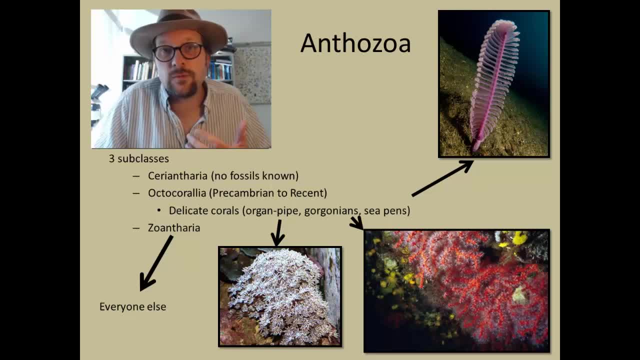 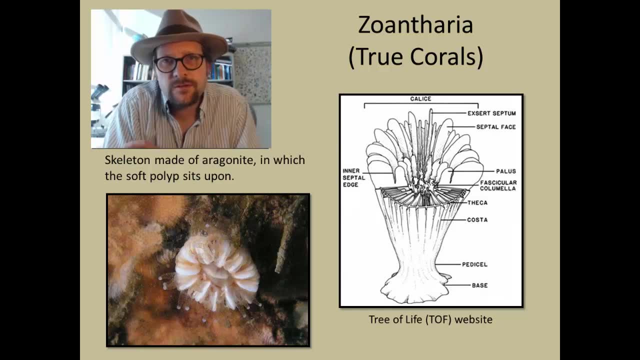 their colonies form hard skeletons and the major reefs of the ocean. They are also called true corals. Their skeletons are made of aragonite, in which the soft polyp sits upon. These cups are called corallium, which house a number of septa that are arranged radially. 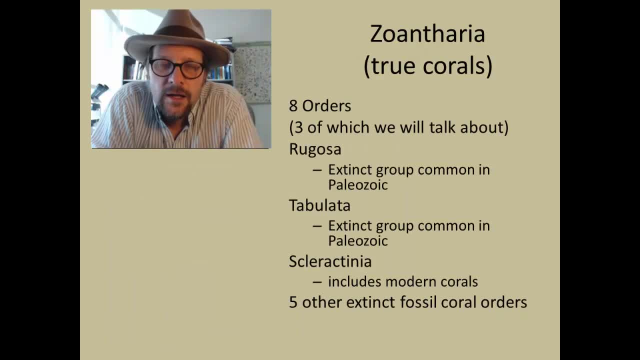 in multiples of six. There are eight orders of Zooanthrea, but only three will cover in depth in this class. The Rogosa and Tabulata are both extinct groups with a fantastic fossil record in the Paleozoic. Both groups become extinct at the end of the Permian. 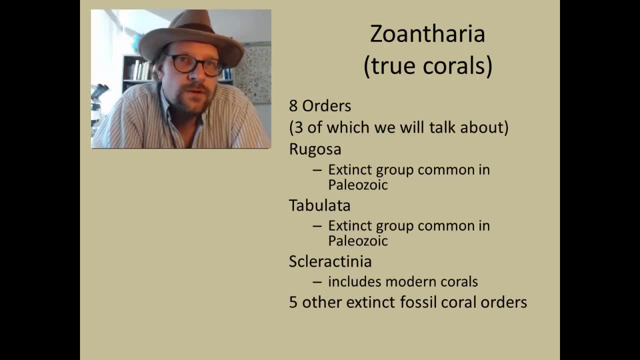 The Scleractinian appear in the Triassic and are known today representing the more common corals found in modern coral reefs. Each of these groups are distinct and easily recognized from fossil records In the Paleozoic. both groups become extinct at the end of the Permian. 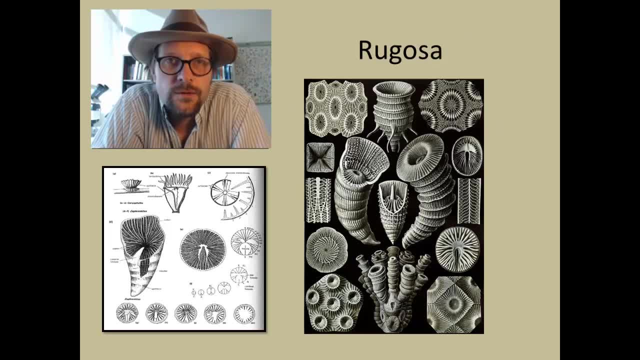 The Scleractinian appear in the Triassic and are known today, representing the more common corals found in modern coral reefs. Both groups become extinct at the end of the Permian. The Rogosa are horn-shaped corals. 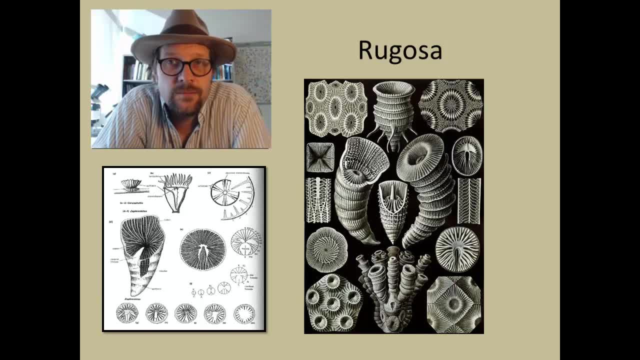 They exhibit a bilateral symmetry around a series of septa that expand out of a horn-shaped skeleton that supported a single polyp. The cup shape, or callus, held the basal ectoderm layer of the polyp. The outer part of the horn is covered in epithecia or calcareous skin, while the internal septa 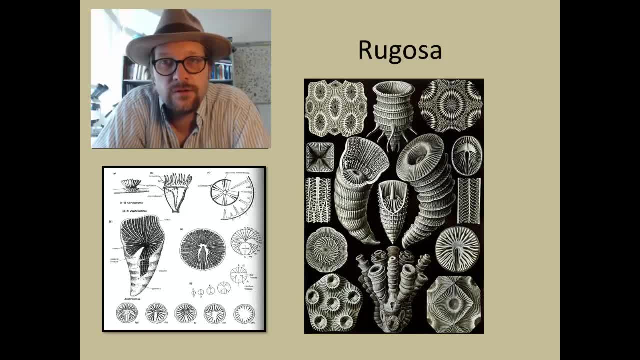 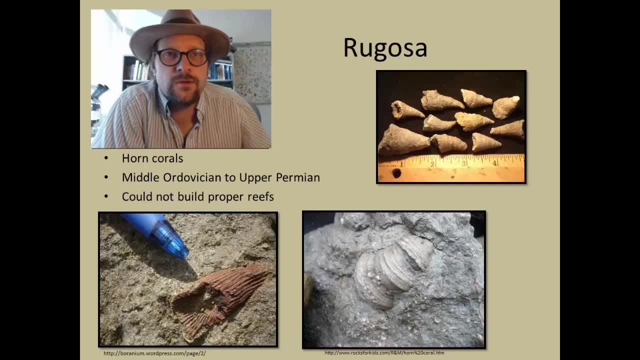 provides a method for identification and classification of various groups of Rogosa. Rogosa are known from the Middle Ordovician to Late Permian and, unlike many other corals, do not form real proper reefs. They are mostly solitary, although colonies are known in the fossil record, in which various 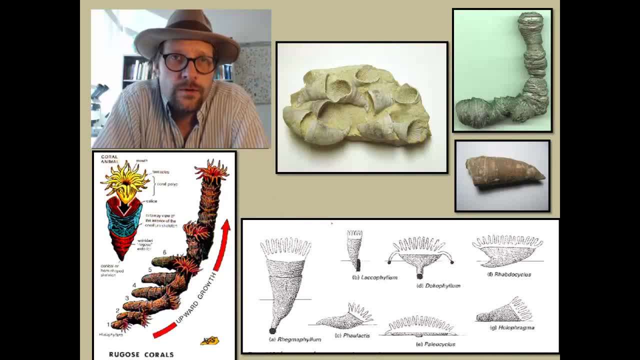 polyps would grow in close association. Rogosa corals expanded through asexual reproduction, through budding and increasing the skeleton as the individual polyps matured. These buds would form within the calyx by axial split or by budding along the periphery. 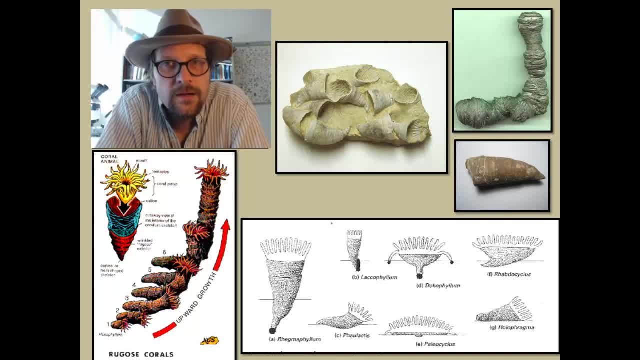 of the calyx or by lateral increase, fully independent of the parent. callus Rogosa also show a pattern of rejuvenansis, where the polyp would grow through periods of starvation and regrowth that likely reflect changing environments and the ability for. 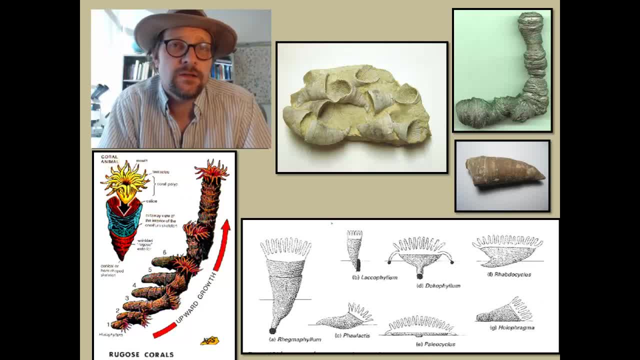 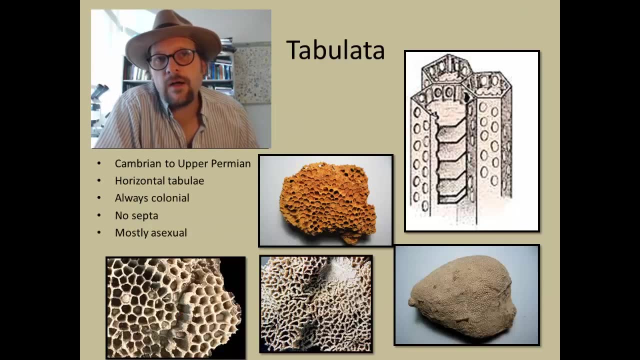 the corals to become more dormant during harsh times and enjoy growth during better times. The Rogosa corals show a trend to grow upward to attain an advantageous position in the water column. The next well-represented coeloteds is called tabulata from the Cambrian to therm ej ang. 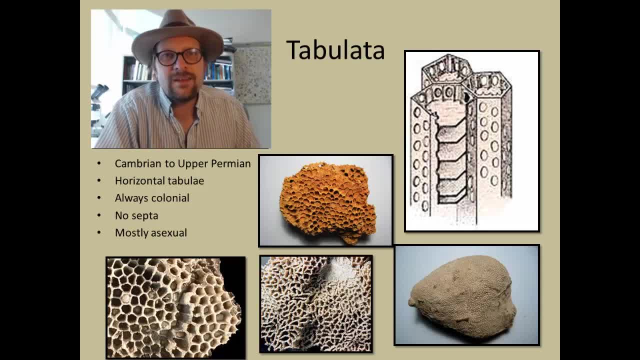 perh me anand exhibit horizontal tabula and, unlike the Rogosa, are colonial and lack septae. They grow through asexual budding, forming broad talons and short Listen wascemi- broad colonies of polyps within a skeletal structure called a corallium. 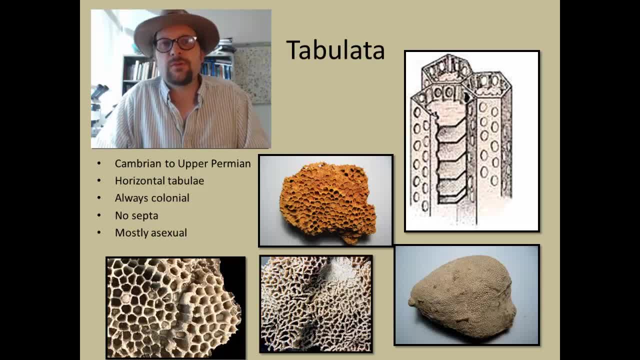 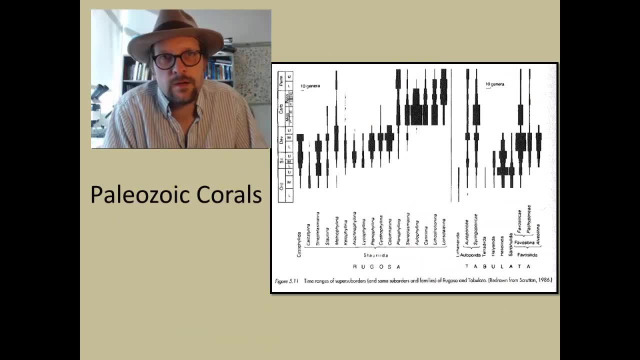 They can bud on the periphery or emerge between these corallates separating across the ocean floor. Both the Rogosa and Tabulata were diverse during the Paleozoic and both became extinct at the end of the Permian-Triassic boundary, attesting to the massive extinction that wiped 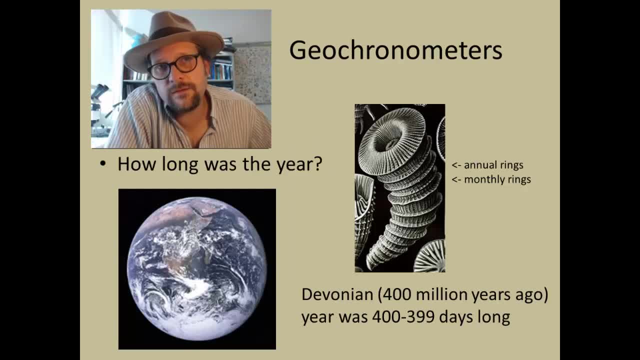 out all the corals living at that time. Another aspect of studying fossil corals is that they can be used as geochorometers. The annual and monthly rings on the Rogosa horn corals can be used to calculate the length of a year in the distant past. 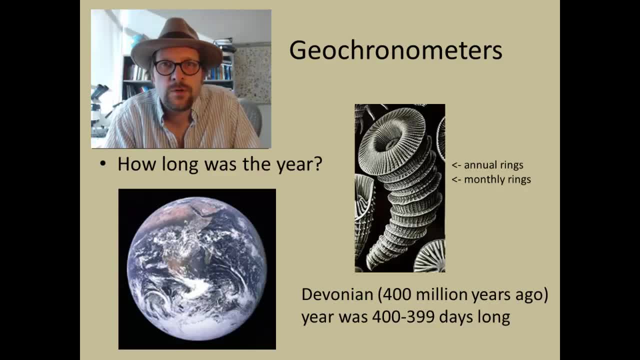 For example, based on Rogosa corals, 400 million years ago in the Devonian, the year was about 400 days long, With much shorter days. Eventually, in the far future, the Earth's rotation will continue to slow down and eventually. 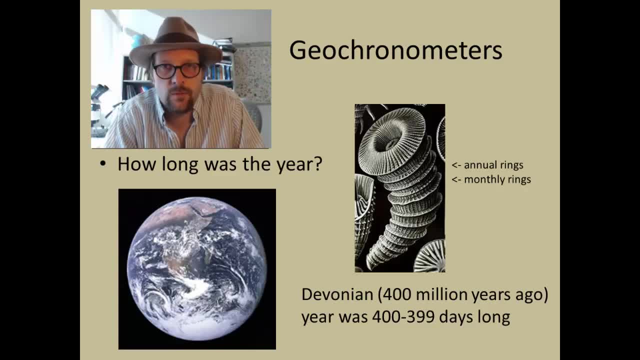 it will match the orbit of the Moon and hence a year will last 24 days. But don't worry, this will not happen. for many billions of years, The inertia of the Earth's orbit will continue to rotate the planet, with only the Sun and 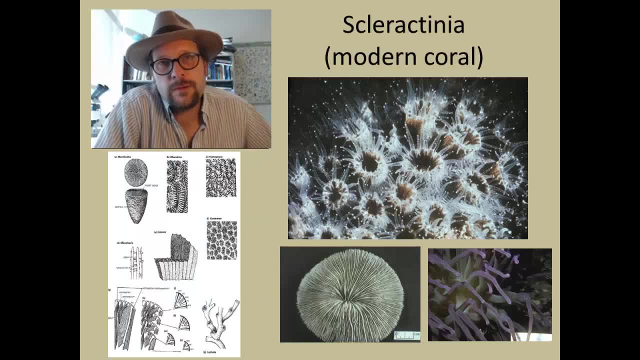 Moon slowing it down slowly. After the Permian-Triassic boundary, modern corals appear in the mid-Triassic: The Sclerotinian Corals. Sclerotinian corals secrete an eragnetic skeleton with septa in multiples of 6.. 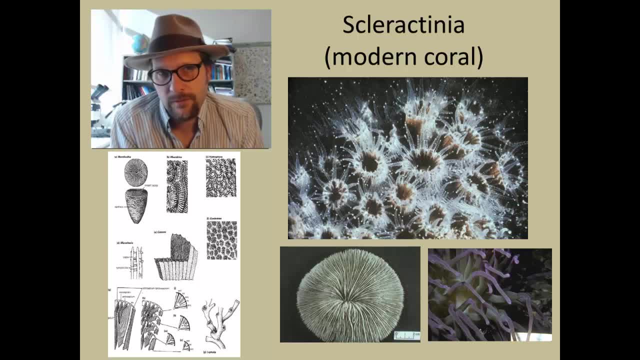 After the first proto-septa grow, they expand to 12, then 24.. This star-like pattern of septa quickly distinguishes them from Rogosa, which are bilateral in their septa formation. Sclerotinian corals are colonial. 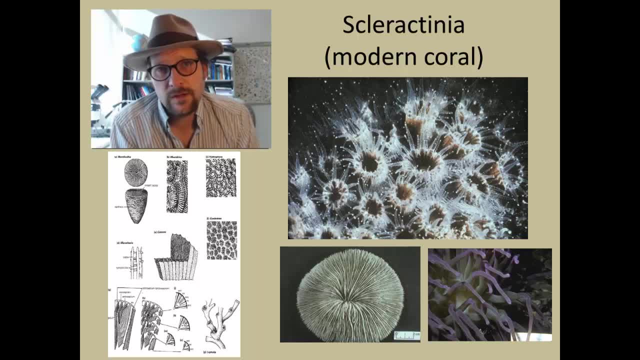 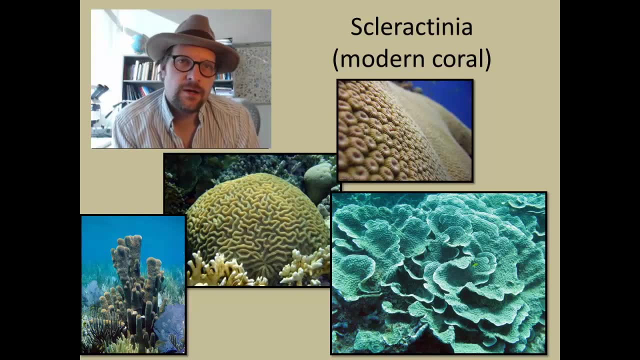 Hence they resemble the tabulata corals. Sclerotinian corals grow through asexual budding of the polyps, but also sexual reproduction by excreting sperm and eggs into the water. Sclerotinians likely arose from soft sea anemone but began secreting a hard skeleton, and hence 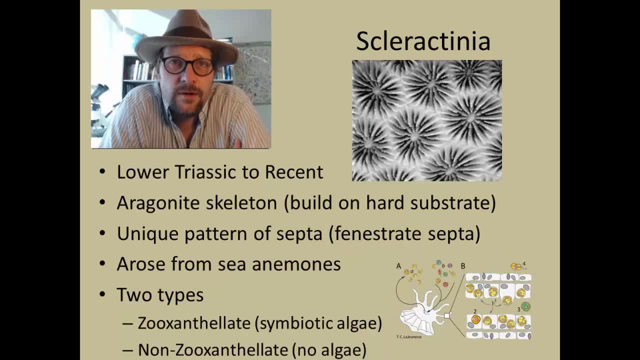 became very common in the fossil record. There are two types of Sclerotinian corals: the Zoonanthia and the Nonzoonanthia. The Zoonanthia is a type of coral that is very common in the fossil record. 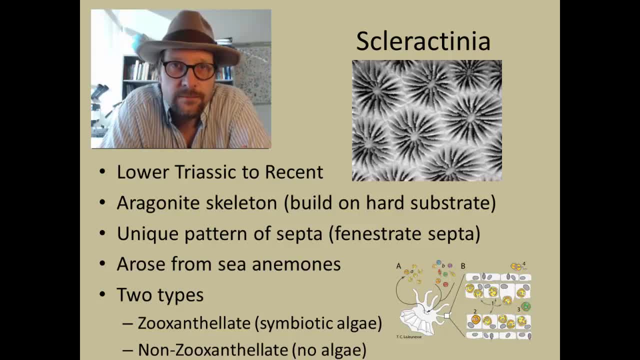 The Zoonanthia contains symbiotic algae, a type of dinoflagellate, which are grown on the coral by photosynthesis and then are eaten by the polyps. This food is about 95% of the food for the polyps. 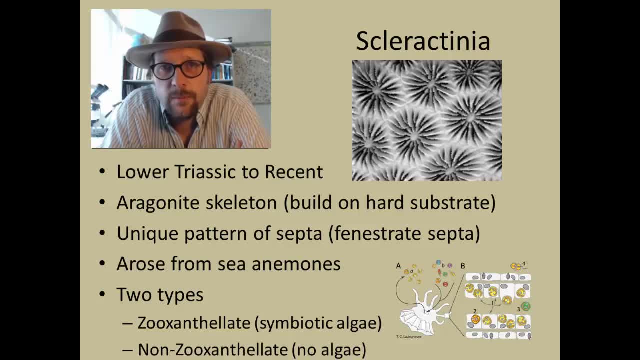 The algae also produces oxygen, which helps the polyps grow. The Zoonanthia corals can also be found in the coral. The Zoonanthia corals can also be found in the coral. The Zoonanthia corals can also be found in the coral. 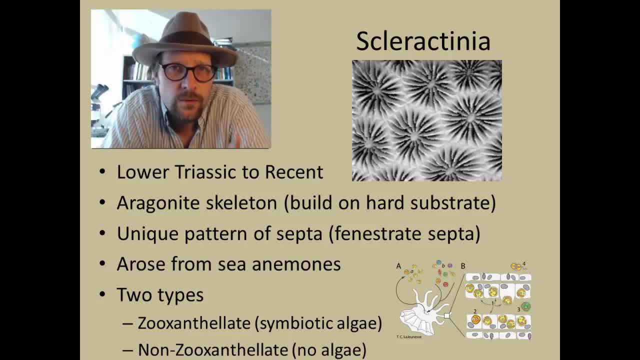 The Zoonanthia corals can only grow in the photic zone and are rarely found below depths of 90 meters. Most of them are shallow waters around 50 meters. The Nonzoonanthia corals can grow at much deeper depths, and those are the ones that 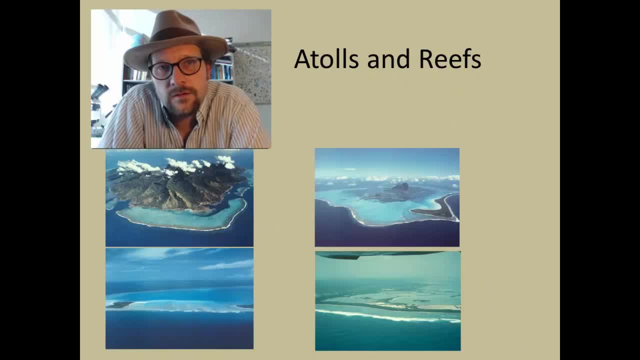 lack the symbiotic algae Zoonanthia sclerotinia. corals are one of the major reef building organisms on the planet Today. they can form atolls and reefs. They are home to an incredible diversity of life. These reefs are resistant to waves and provide for shallow lagoons which offer a protective. 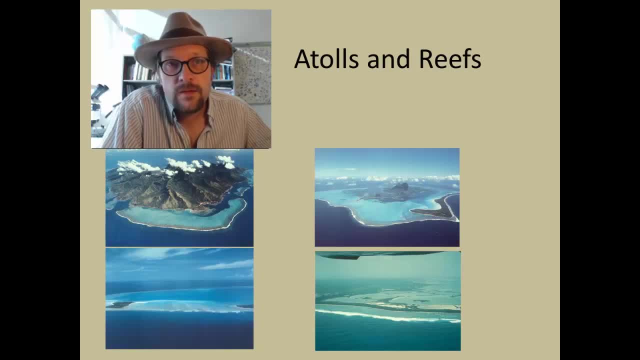 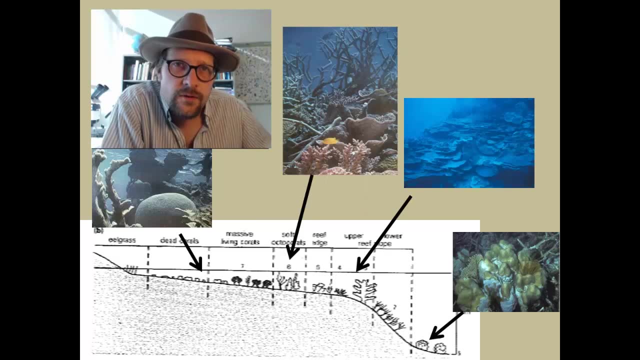 habitat for many marine organisms. These reefs can become incredibly thick deposits of carbonate as thick as 2 kilometers. Study of living corals also gives us insight into the habits along the margins of the coast By studying the types of corals along the shoreline. 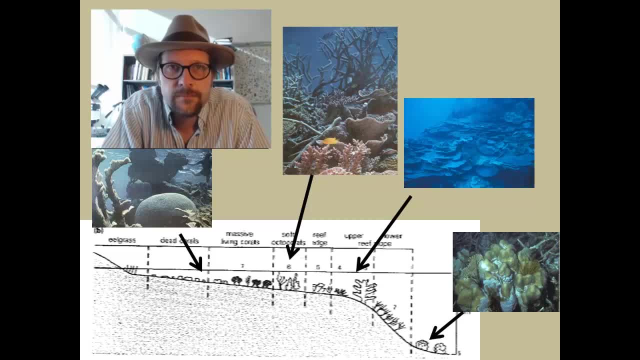 We can reconstruct the changes to the depositional environment. Where corals are subjected to dropping sea levels, they can die and erode, while corals within the photic zone flourish as long as they remain in the water. Such patterns can be important for the exploration of petroleum reservoirs associated with ancient 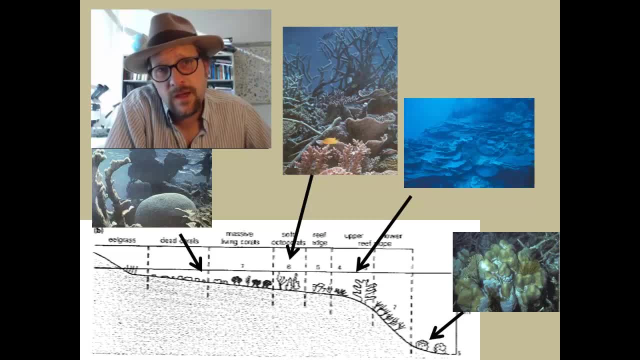 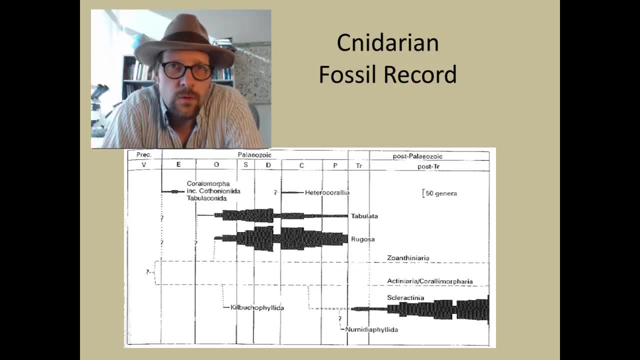 coral reef complexes, such as those in the Permian Basin of Texas and Saudi Arabia. 2. This diagram shows the geological ranges of the various fossil coral groups, with modern sclerotinians appearing in the mid-Triassic and as the sole large group of corals that.